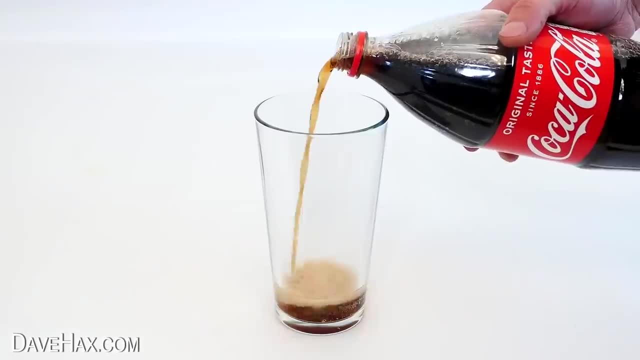 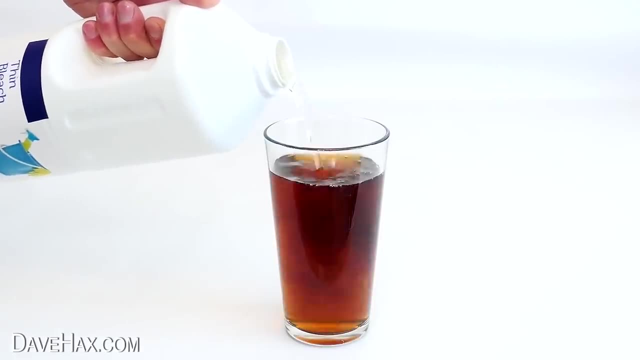 Here's a great one to start. How do you make a Coca-Cola drink transparent? Well, use bleach. Watch what happens when I top up the glass. You can see the colour being stripped out of the Coke. Give it a mix and leave it to sit for a few minutes. 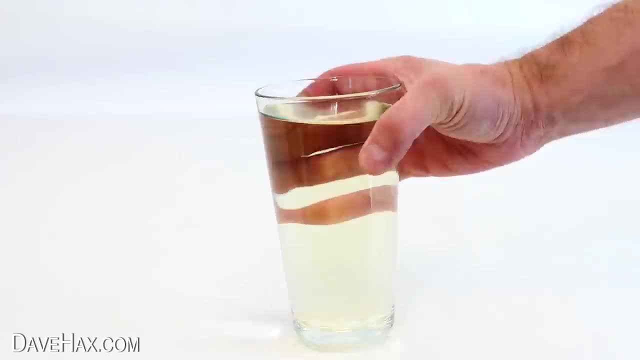 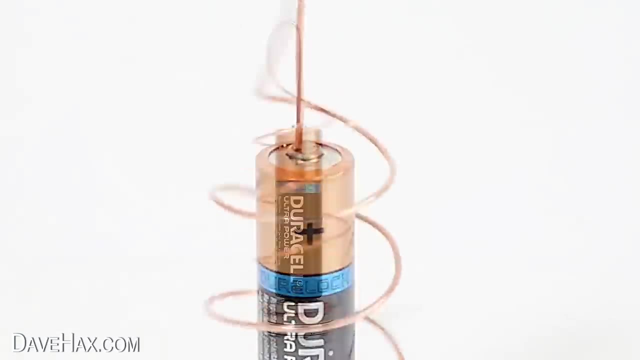 And it turns completely transparent. Crazy huh. Of course, make sure you don't drink it and dispose of it carefully. For the next one, I'm going to show you how to make a really simple homopolar electric motor. It's really easy to make. 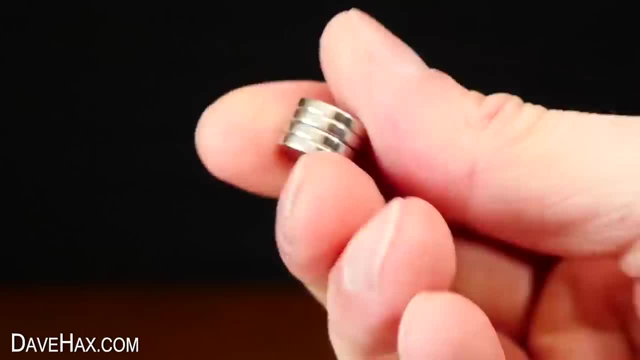 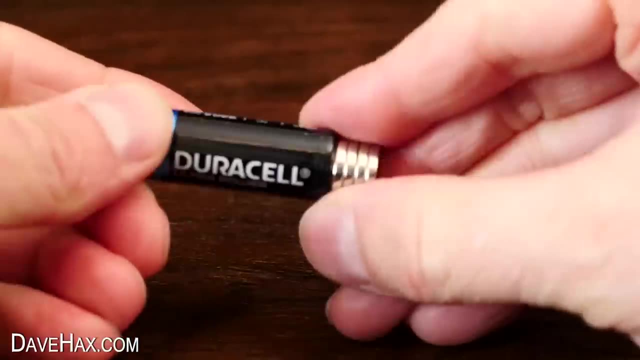 All you need is an AA battery, circular magnets and some copper wire. So to make the motor you'll need some copper wire To make the motor. we attach the magnets to the base of the battery, Then take a short length of the copper wire. 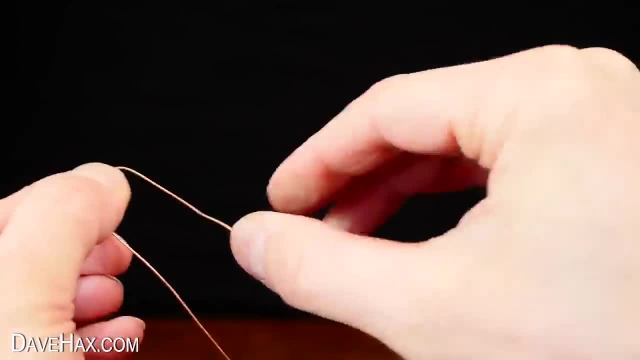 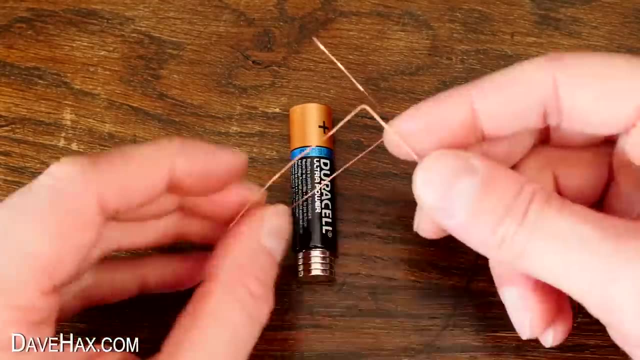 Fold it in half, Then fold it back on itself like this. Next we need to measure it alongside of the battery And fold the wire over at the same length as the magnets, Then form a loop at each end, so it looks like this. 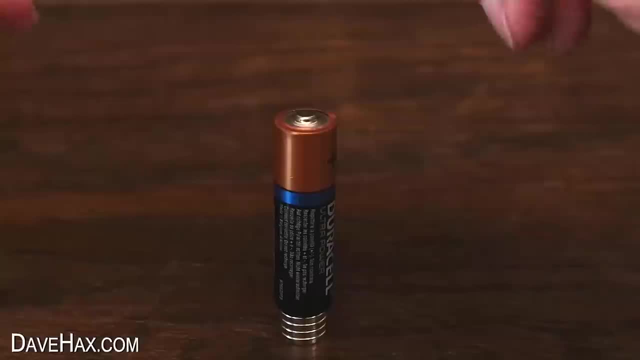 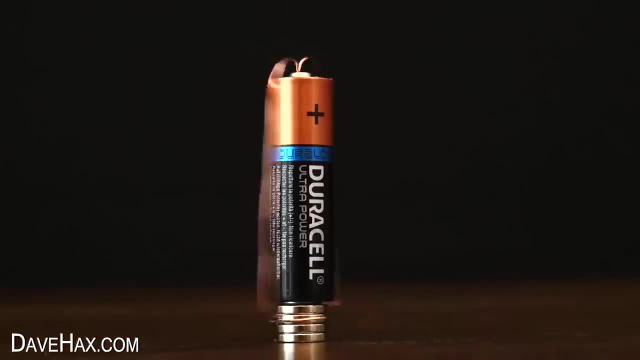 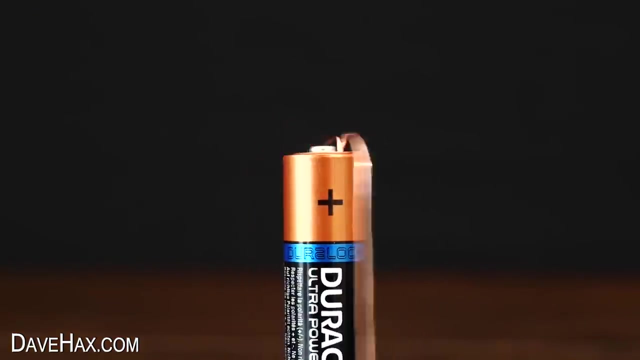 This loop will hug the magnets at the base, Slide it over the battery and balance it on top And off it goes. Look at it spin. We've made our motor. You do need to make sure the copper is well balanced so it doesn't fall off. 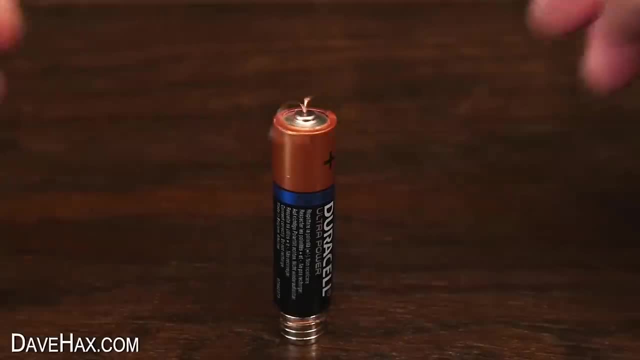 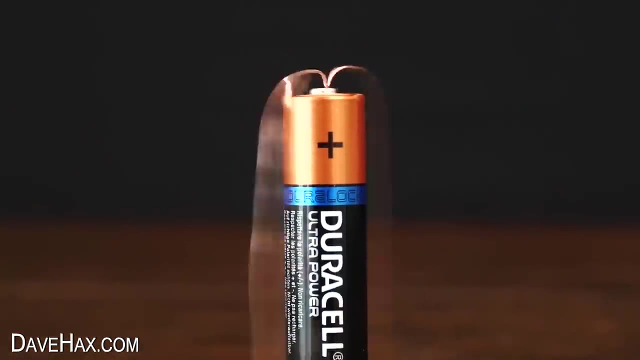 So the battery causes current in the wire which interacts with the magnetic field from the magnets, And that's what causes the wire to spin. You can make them out of different sized batteries. Here I'm using a slightly larger battery And here's one with a tiny button battery. 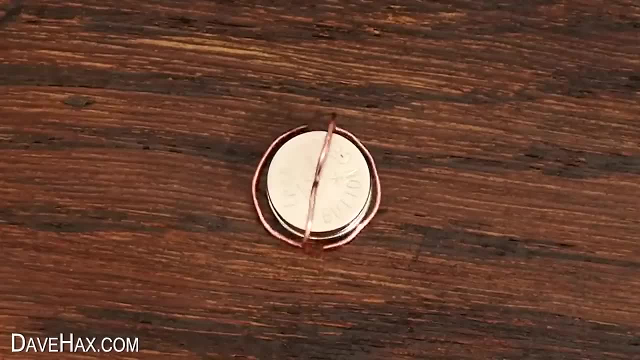 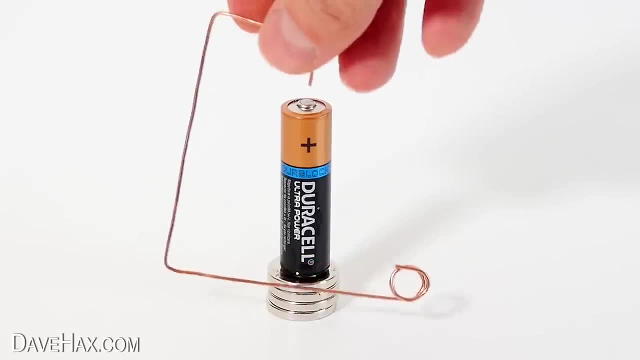 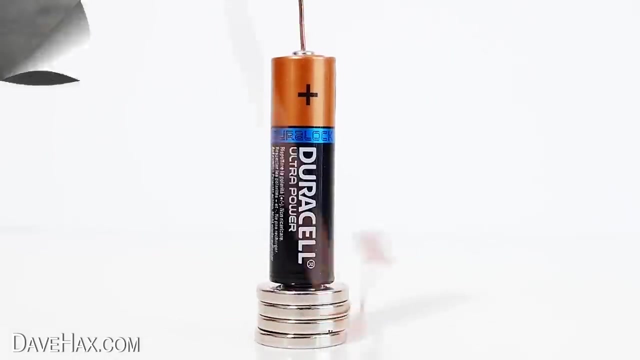 Order the battery- And here's one with a tiny button battery- Or try experimenting by making different shapes of wire. I really like this spiral design And this counterbalance one too- Just remember it does need to balance. For the next one, I'm going to show you a really cool trick you can do with dry wipe marker. 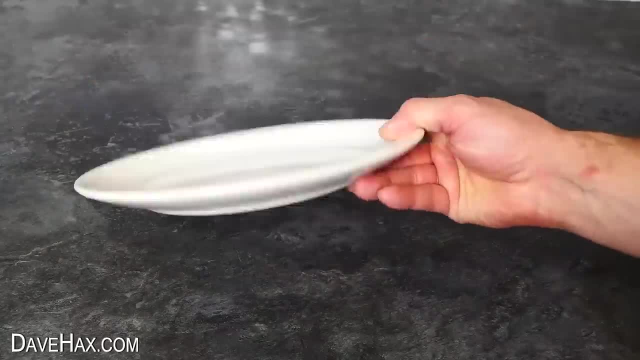 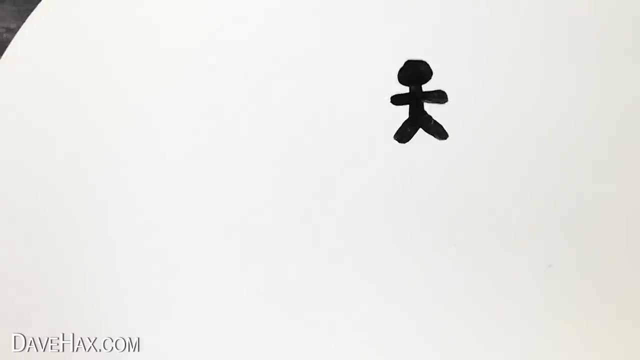 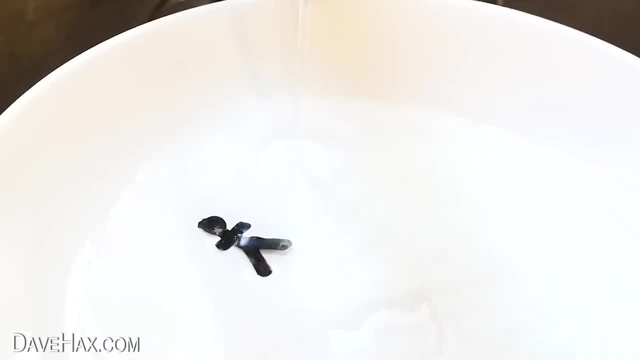 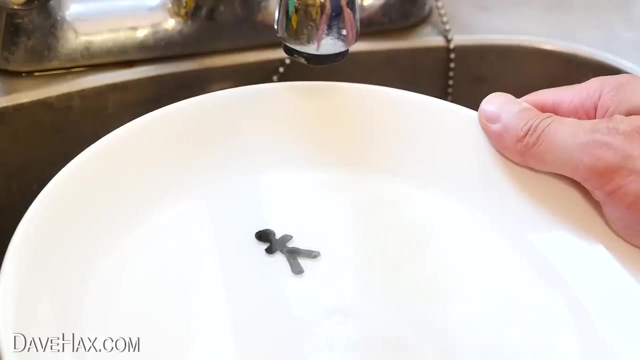 I'm drawing a stick man. I'm drawing a stick man. I'm drawing a stick man. Now look what happens. when I hold the plate under a tap And slowly dribble water along side of the stick man, He starts to lift off the plate. 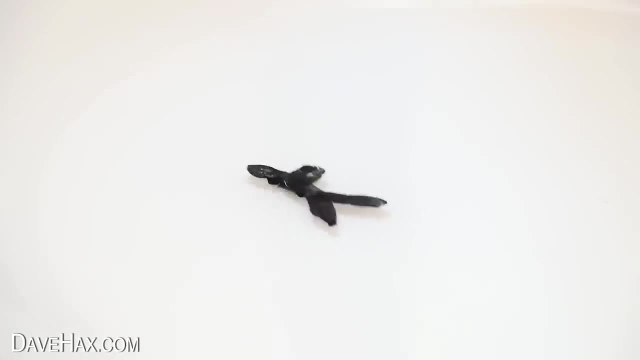 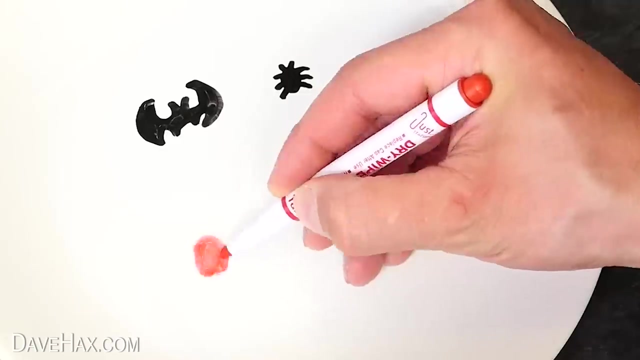 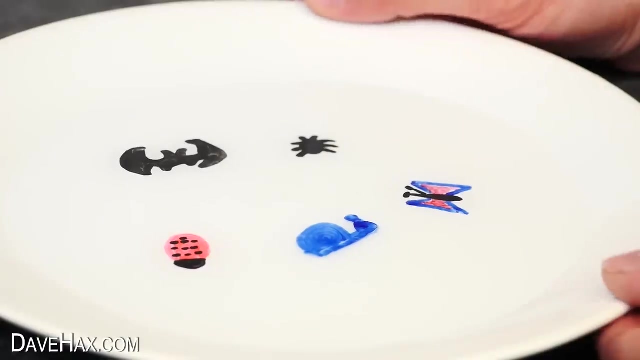 Then breaks free And floats on the water. Let's see it from another angle. You can see he's still partially attached to the plate. Then, with a bit of a wobble And a shake colours on the same design, Add water. then slowly give the plate a wobble and watch as they break. 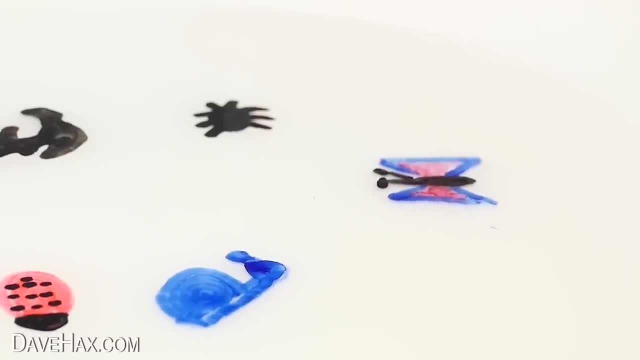 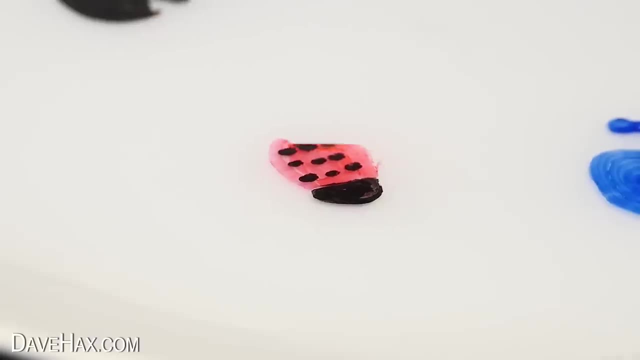 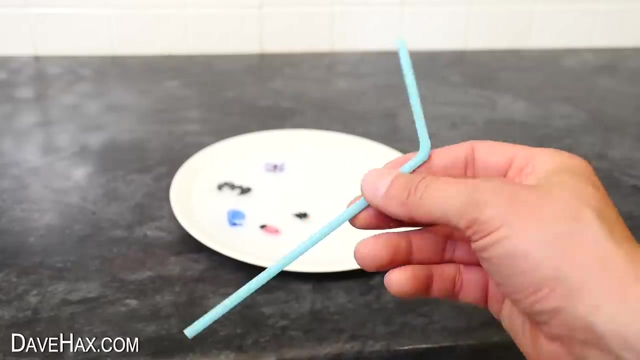 free. You can see the snail is free, there goes the butterfly, then the bat breaks free and the beetle and finally the ladybird. You can carefully move them around with your finger. or what's really cool is taking a drinking straw and blowing them around with that. For the next one I'm going to 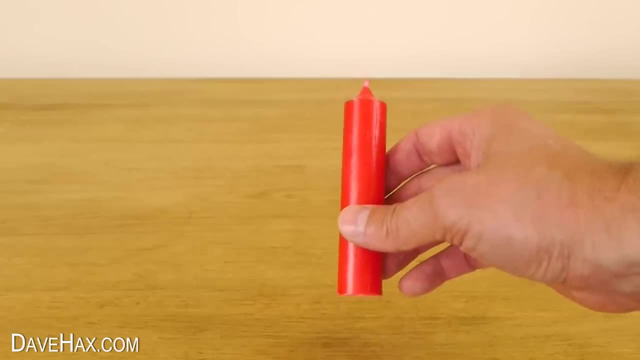 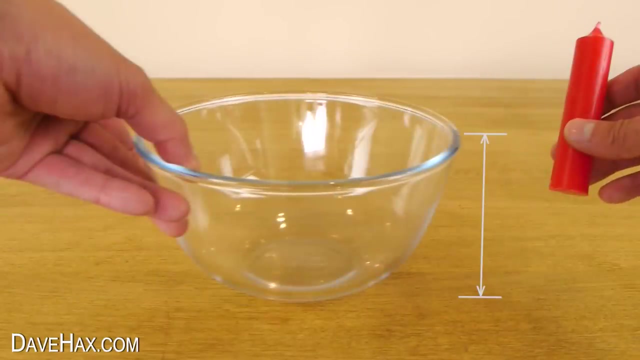 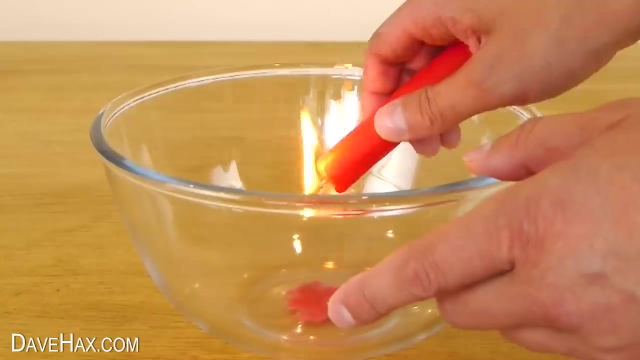 show you how to burn a candle under water. My candle measures about 22 millimetres in diameter and I've cut it so it's roughly the same length as the depth of this bowl. I started by lighting the candle, dripping a good puddle of wax into the bottom of the bowl. then I extinguished it. 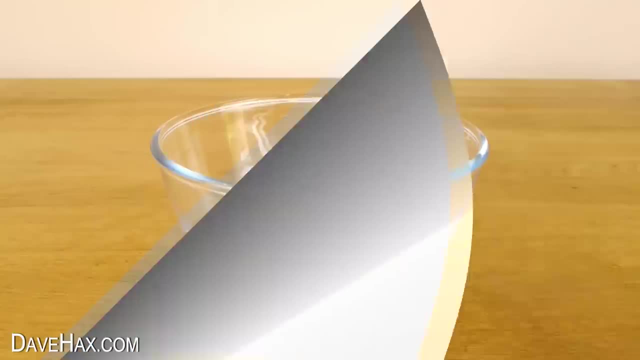 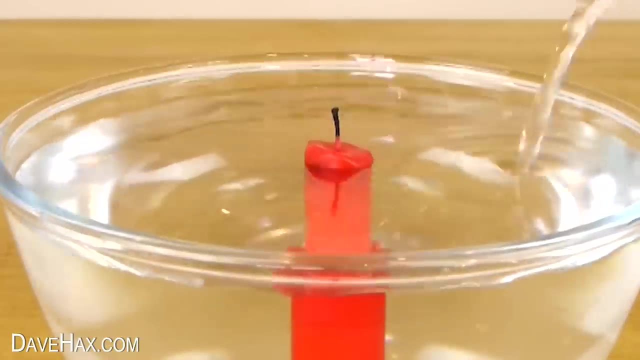 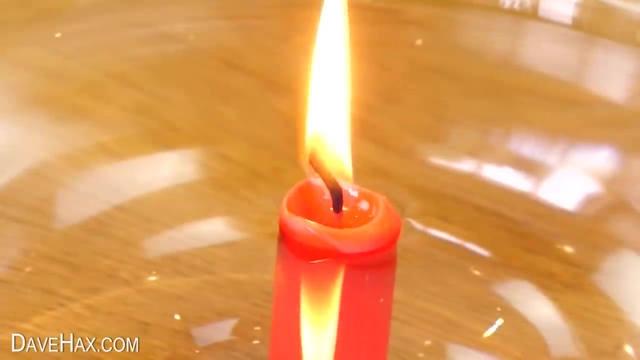 and stuck it down into the molten wax. Let it dry for a few minutes, and then I'm going to fill up the bowl with water until it's just underneath the bottom of the candle. Let the water settle, then go ahead and light it. I'm speeding up the video now so you can see what. 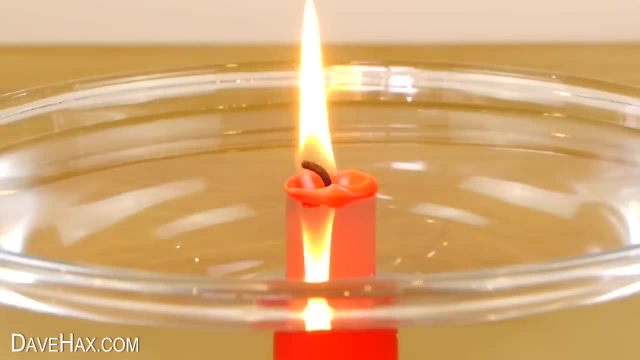 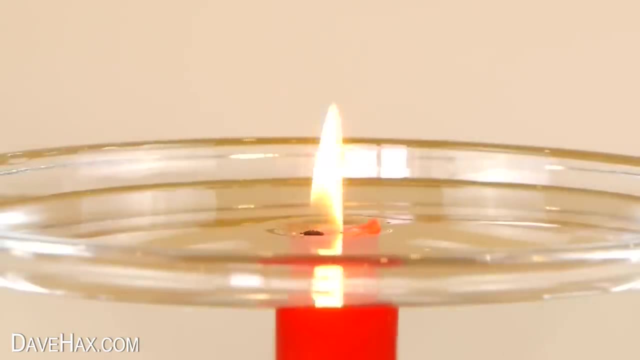 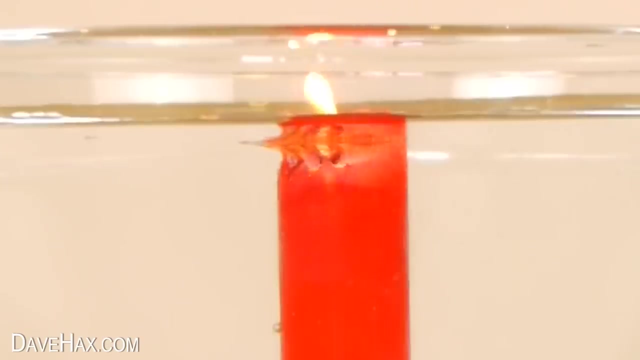 happens. As the wax burns, the water keeps the outside of the candle cold, so it doesn't melt, and the flame actually drops below the surface of the water. Eventually, though, it does melt through, and the candle will flood, But I used a piece of wire to measure how far the candle had burnt down beneath the surface of the water. 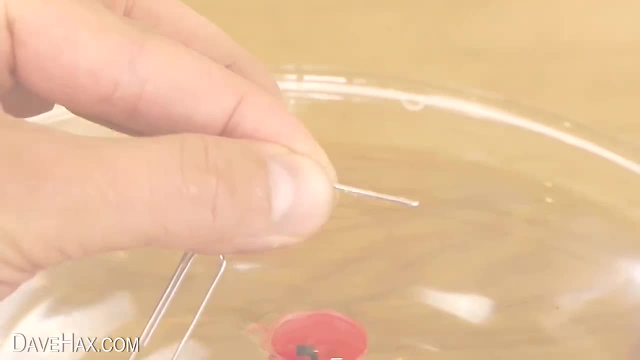 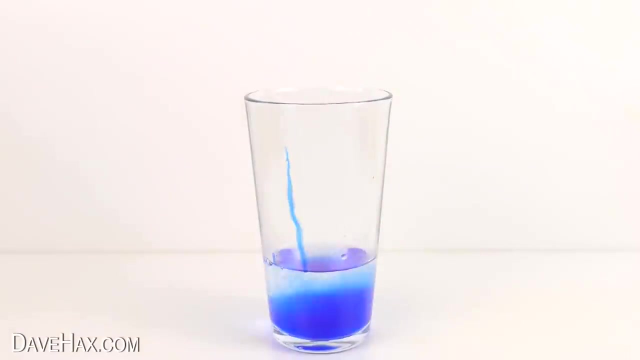 Mine went down about 18 millimetres. In this experiment we're going to learn about density. Start by taking an empty glass. then tip in some water and food colouring, then add some syrup or treacle. I added a little more water to make the layer a bit thicker. Then finally fill up the glass. 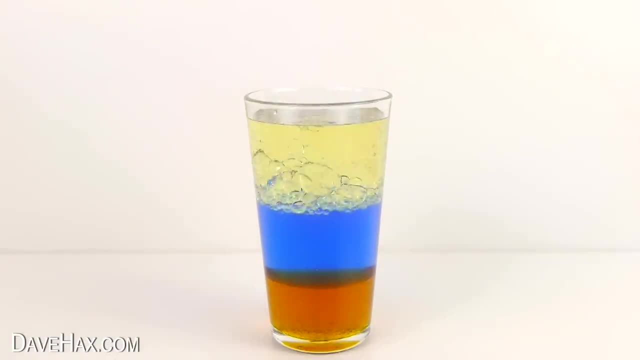 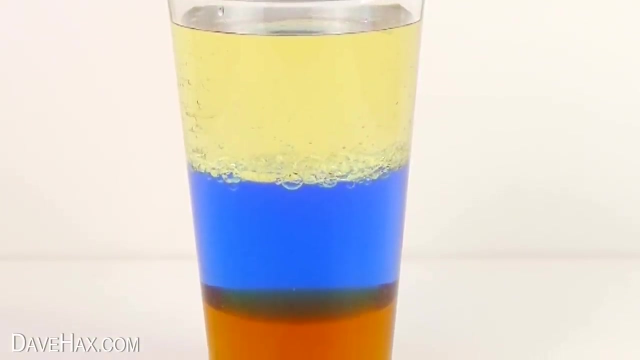 with some oil And leave it to settle for about 15 minutes. As soon as you see the oil on top of it, it's ready to be dissolved. These liquids separate out into different layers because they're different densities and they don't mix. 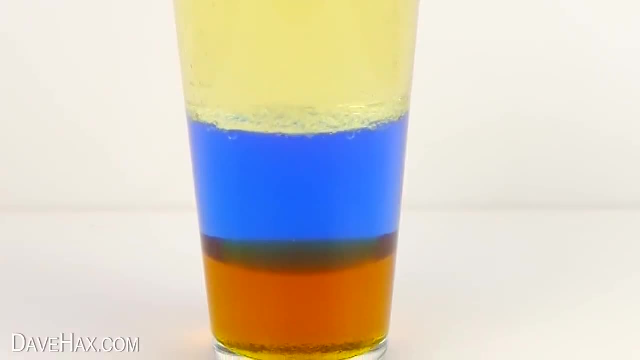 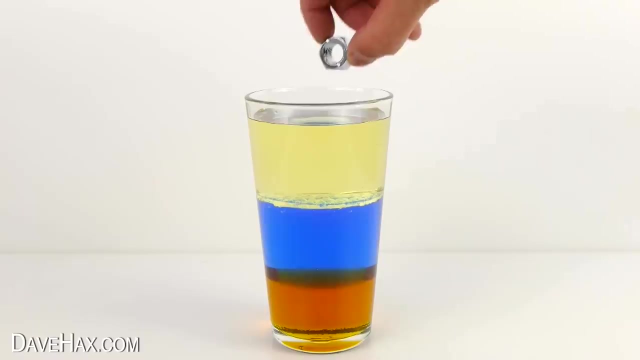 The syrup has the highest density, so it sits on the bottom, the water sits on top of that and the oil, which has the lowest density, sits on the top. Now we're going to try dropping different objects in to see what happens. If we drop this metal nut in, which is really dense, it sinks straight down to the bottom. 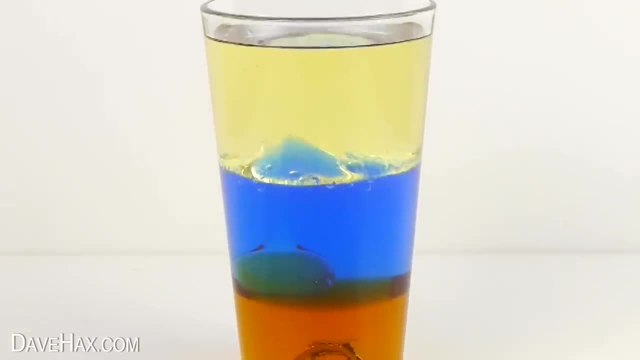 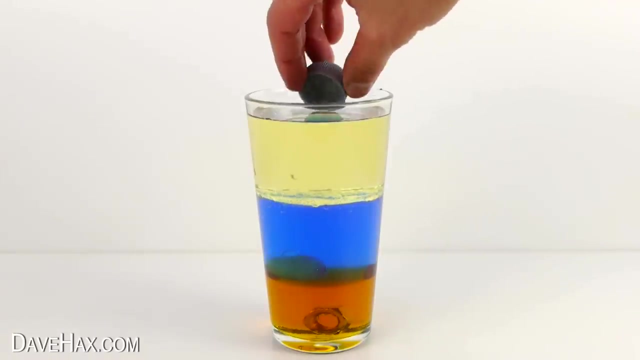 But if I take this grape and drop it in, it sinks through the oil and water and the syrup gets absorbed and breaks up into the bottom but sits on top of the syrup. this is because the syrup is denser than the grape. now if I take a plastic bottle top and drop it in, it slowly sinks through. 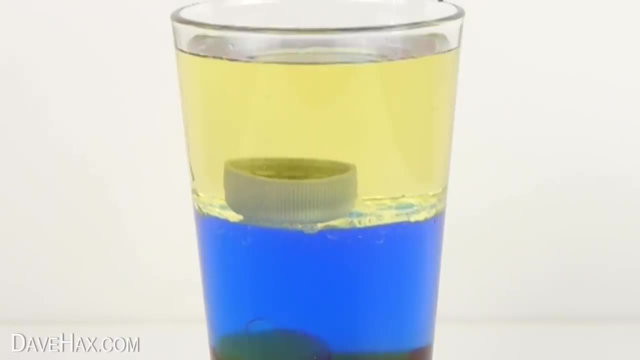 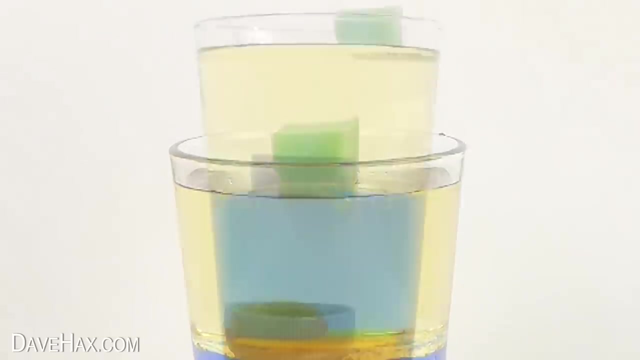 the oil and sits on the water. and finally, if I take this piece of sponge and drop it in, it sits on top. the oil is denser than the sponge. you can try dropping different objects in to see which fluid is denser. for this one I'm. 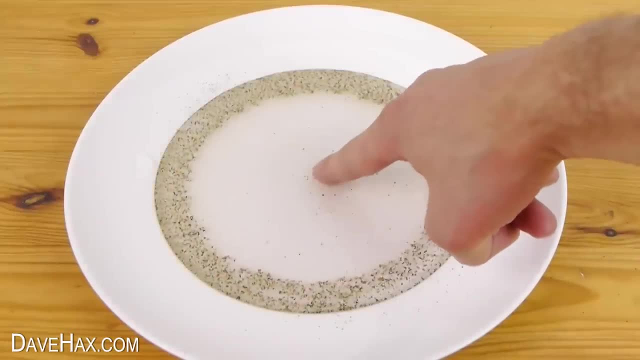 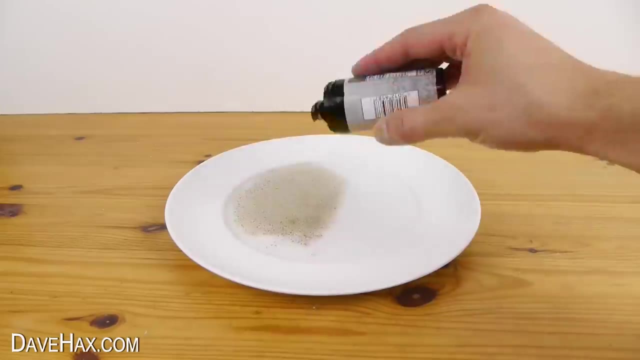 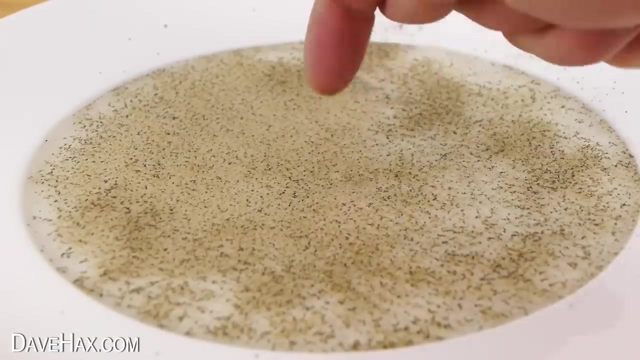 going to show you a really cool experiment with water and ground black pepper. start by taking a plate and pour on some water. then take your pepper and sprinkle a fine layer all over the water, nice and evenly. like this you can see the pepper sits on the surface of the water and if you dip your finger in, 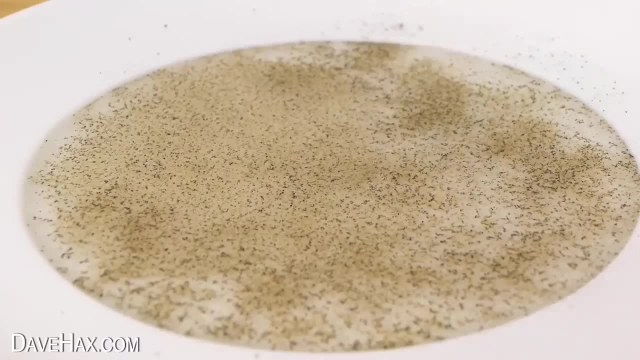 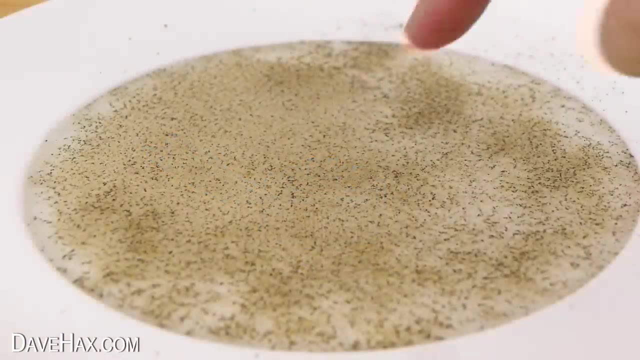 nothing much happens. you might get some pepper stuck on your fingertip, but that's about it. next, take some washing up liquid and wipe a tiny bit on the end of your finger. then try dipping it in the water again. this time, as you can see, the pepper seems to have dried out a little bit, so I'm going to take some. 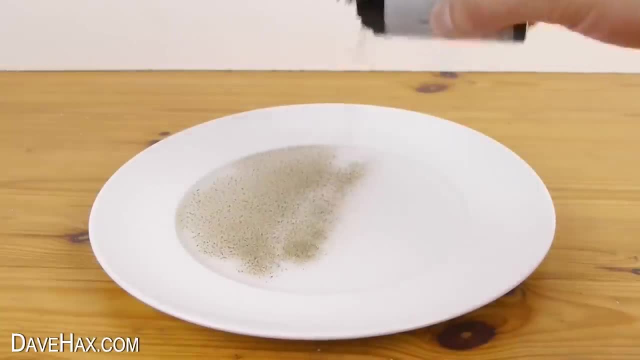 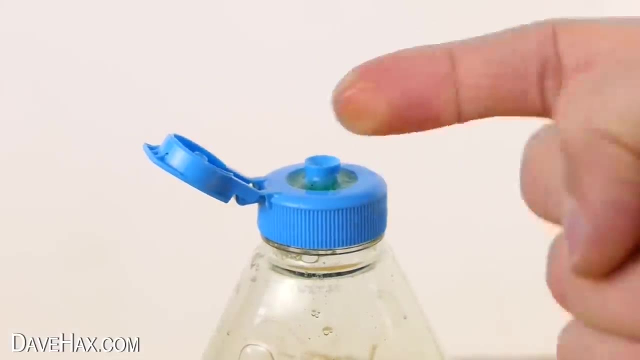 water and drop it into it so it doesn't get on the surface of the water, and then have some more water get on the bottom and if you dip your finger in it again, slowly and gently, this will help the water and come back to the surface. so here's what's happening: the pepper sits on the water because of the high 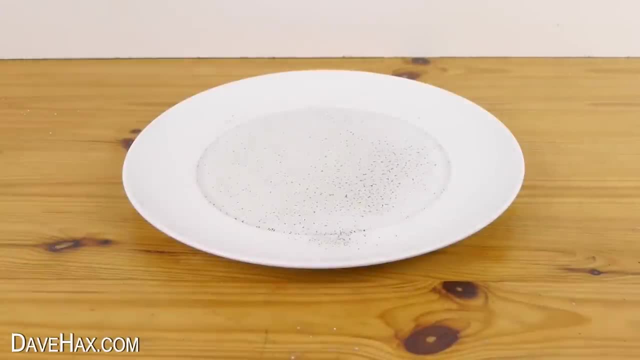 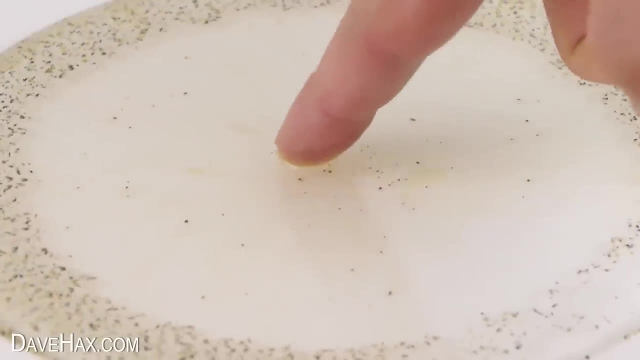 water surface tension. the water molecules are strongly attracted together. when we add a little soap we break down this surface tension and the top layer of water molecules very quickly spread out and carry the pepper animals that we created earlier. I'm just adding a drop of washing up liquid into. 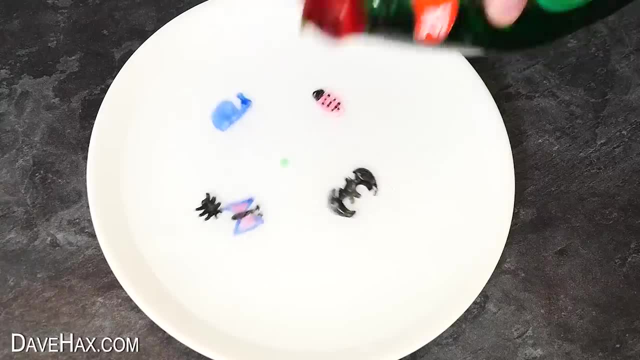 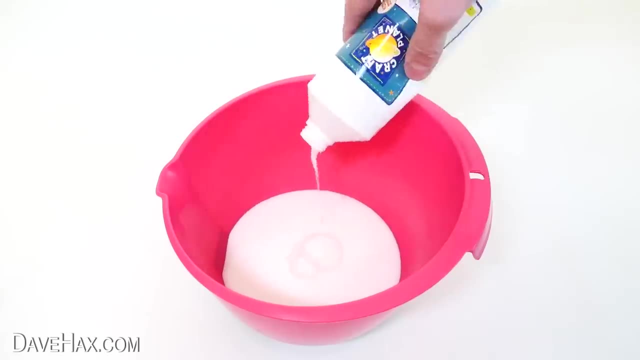 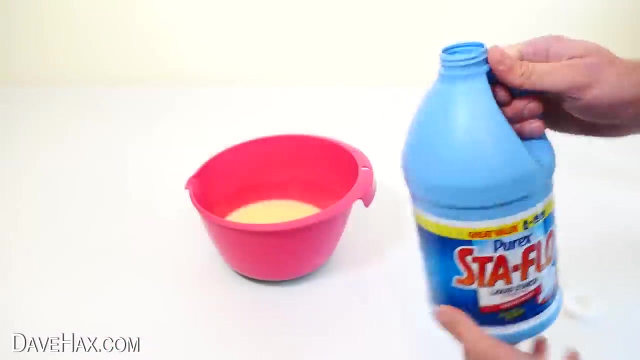 the middle and watch as they shoot to the side. for the next one. I wanted to see what happens if we froze slime, so I made up some slime out of PVA glue, added a bit of water and food coloring and some stay flow liquid starch. I mixed it. 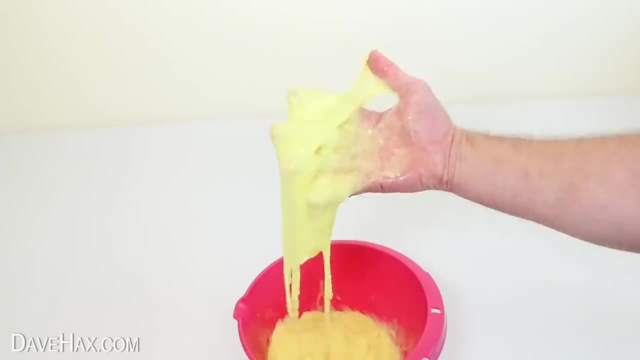 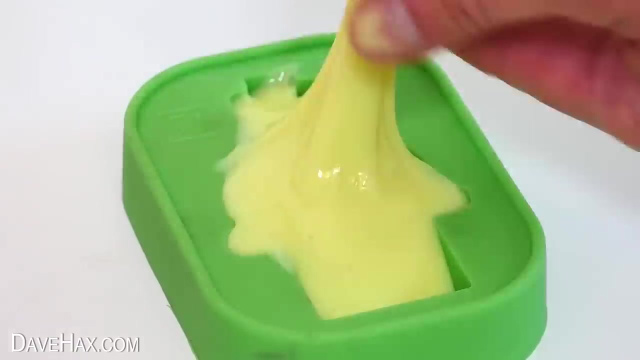 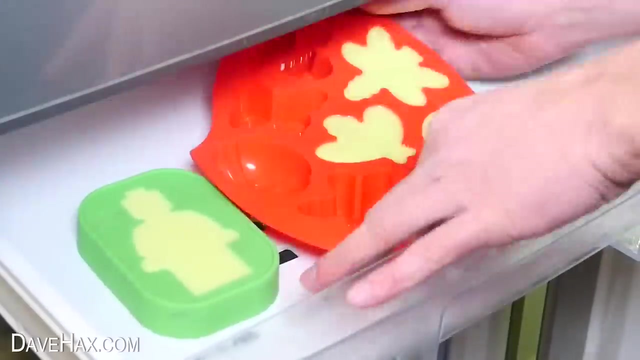 together into this really cool slime. it's really stringy and great fun to play with. but I decided to put it into molds to see what happens if I freeze it. so I filled up this Lego style figure mold and also these bugs, then popped them into the freezer. I left them overnight to freeze, then took them out. 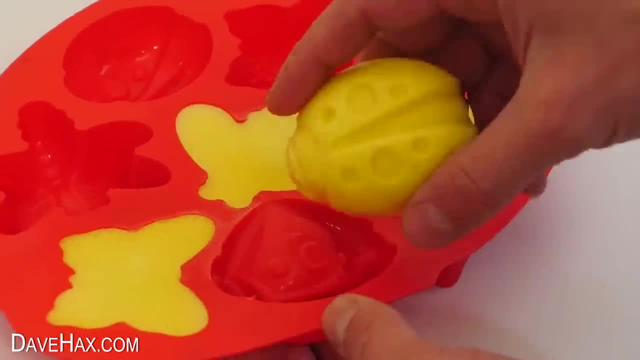 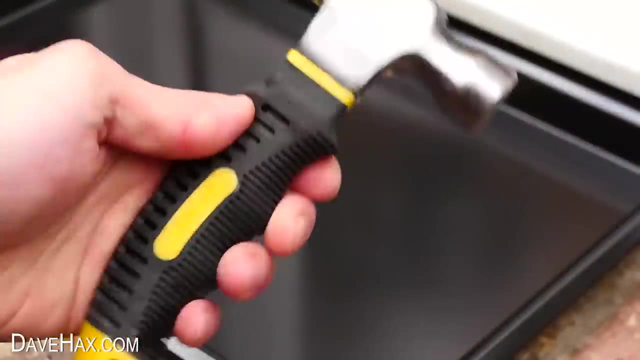 they froze really well, they come out of the molds easily and the level of detail is really good. I decided to try hitting one with a hammer to see if it would shatter. at first it just chipped a bit off and slid from under the hammer. unfortunately, it didn't work out as well as I thought it would, so I decided to try it out and see what happens. 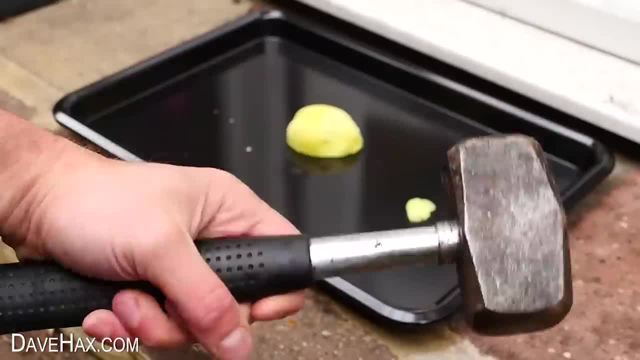 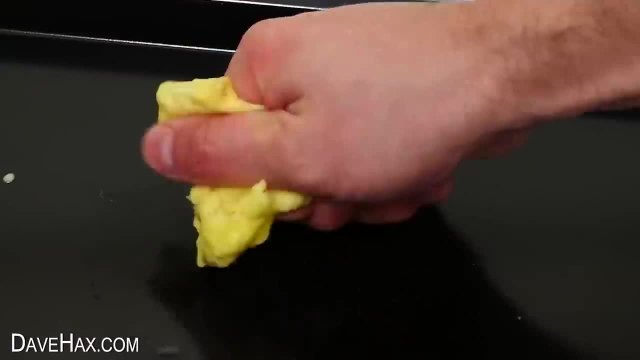 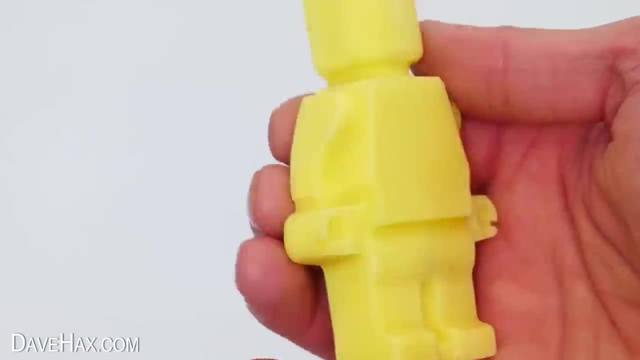 so I tried again with a bigger hammer and it fractured clean in half. as it warms up, it starts to thaw out and you can mold it again with your hands. it returns back to ordinary slime. this figure also came out really well, but I decided just to warm it up with a blowtorch, to melt it back down and 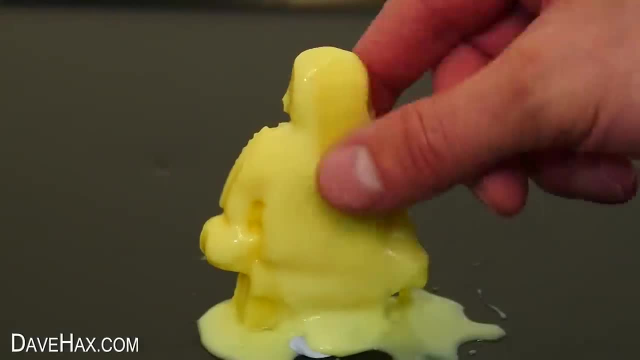 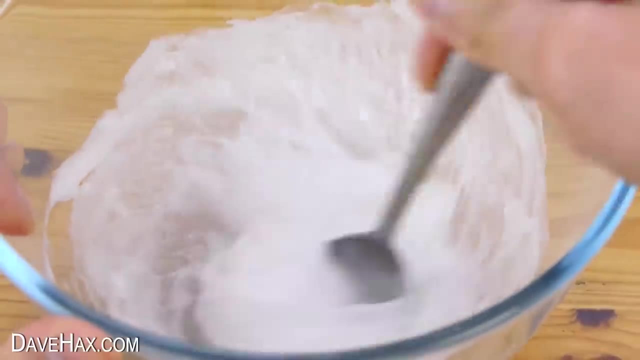 convert it back to slime. but for the next one, I'm making this really amazing magnetic slime. I started with a little bit of glue and then put it into the mold and then I started by making a base slime the same way as before. you could, of course, add food coloring. if you want to make it a color, then to make it. 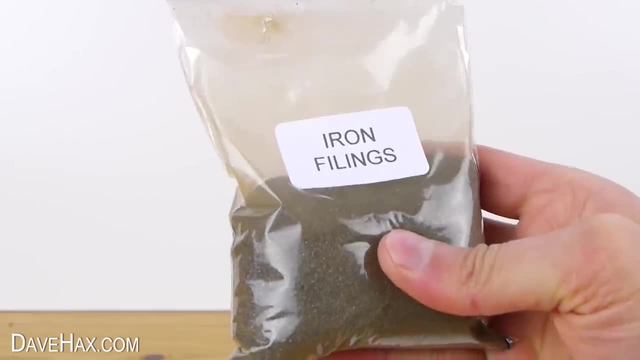 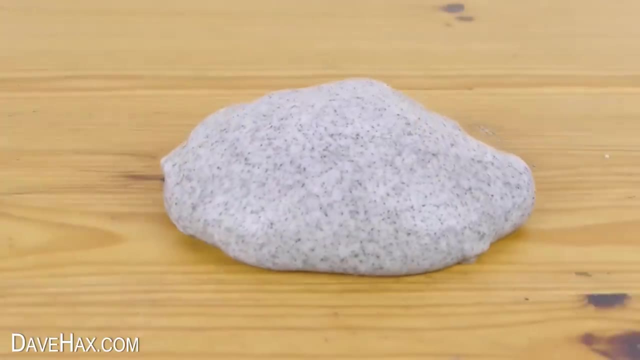 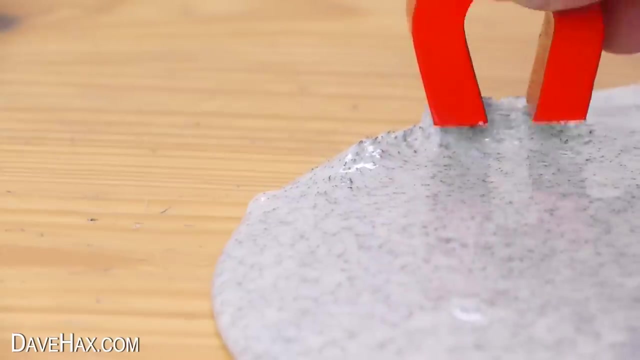 magnetic. I'm adding iron filings. I poured some onto the slime and worked it into the mixture and when it's ready you should have a light grey slime. now take a magnet and hold it close by to see how it reacts. the slime is attracted to the magnet and you can make it move. you've got to be quick or it'll stick to the 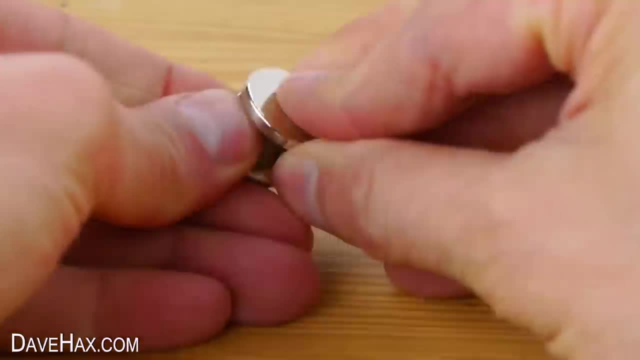 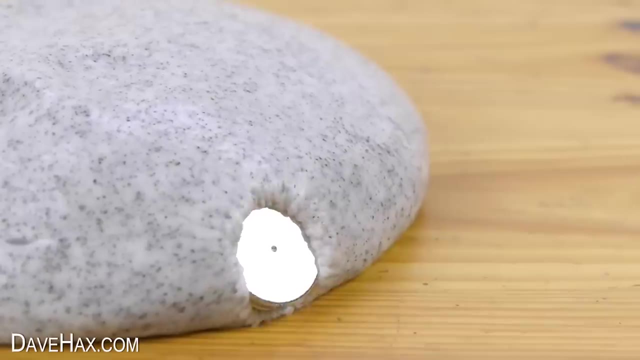 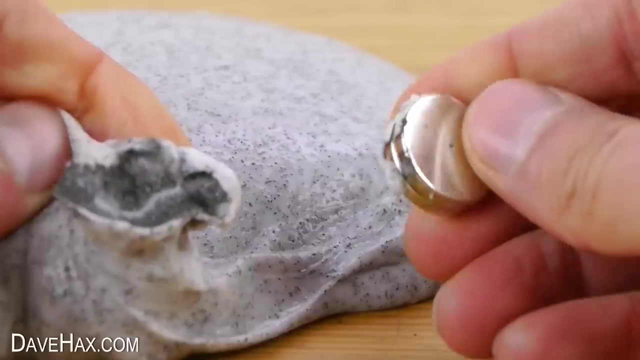 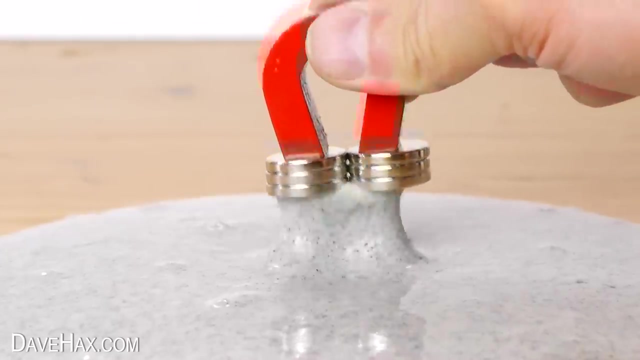 magnet. these neodymium magnets are really powerful. watch what happens when they get stuck into the slime. it kind of just swallows them up. pretty cool, huh. I have speeded up some of the footage so it's quicker to watch. you can stack up magnets to make them stronger and watch what happens: the slime sort of jumps and